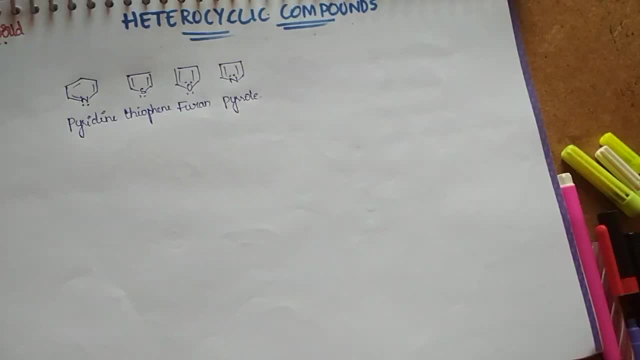 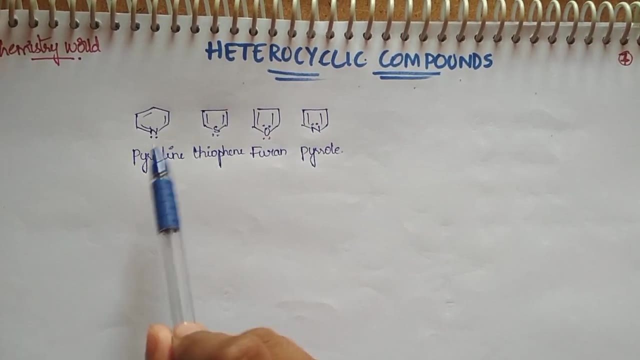 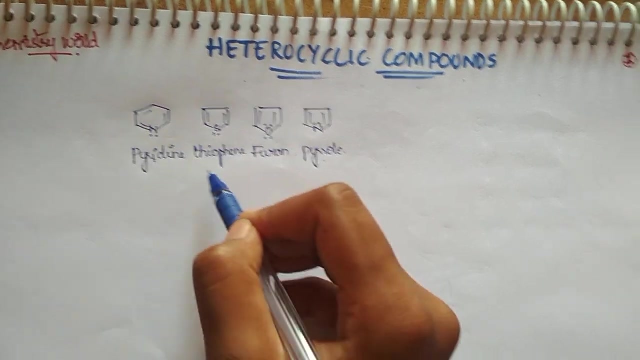 Hello, welcome to the chemistry world. Today I'm gonna tell you about heterocyclic compounds. Okay, so we have the heterocyclic compounds like pyridine, thiophene, furon and pyrrole, But the six membered ring is pyridine and the five membered ring or thiophene, furon and pyrrole. 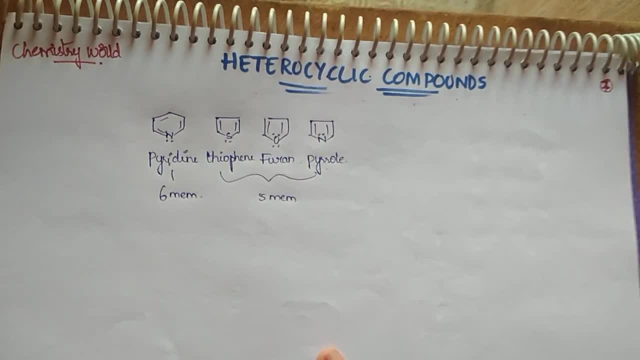 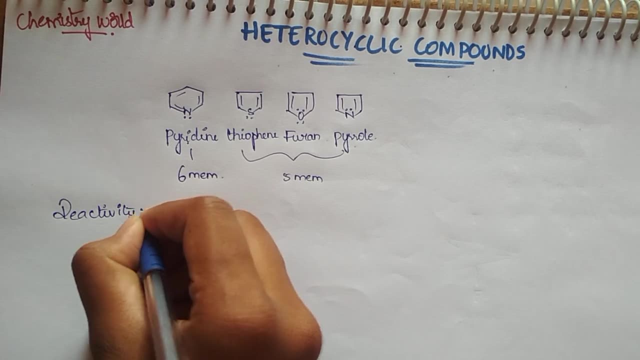 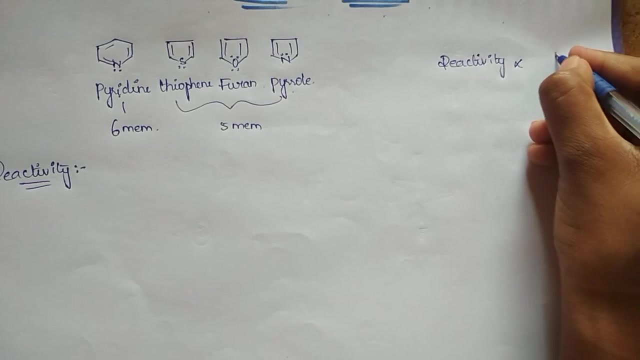 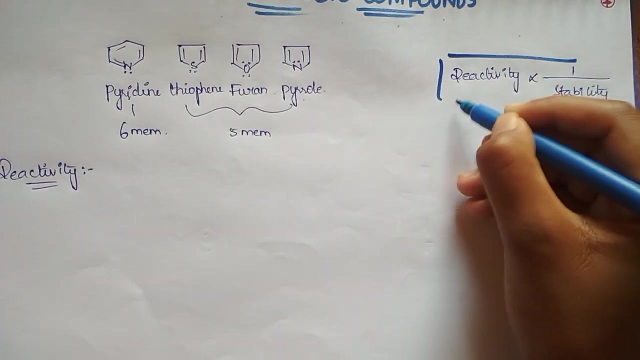 Okay, students, next, First of all, we discuss about reactivity. First of all, you know, the relation between reactivity is inversely proportional to the stability. It is a major concept. You have to learn it quickly, Right, students? It is a major. 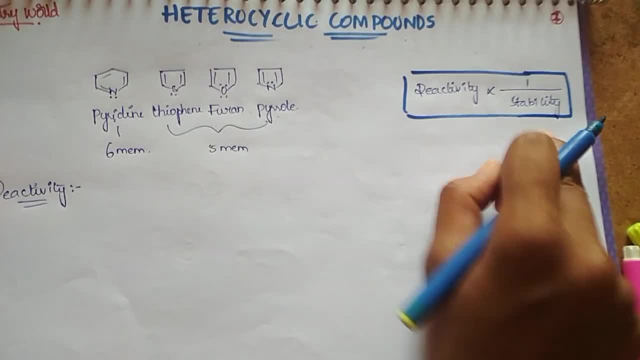 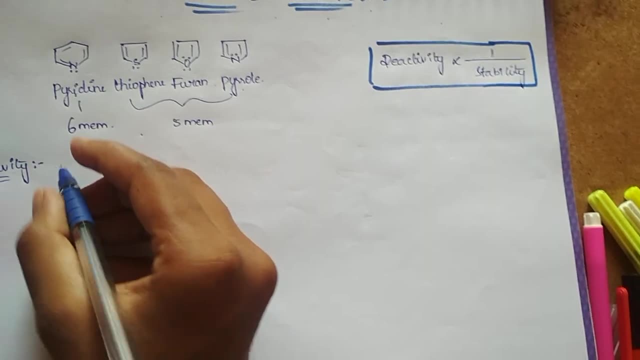 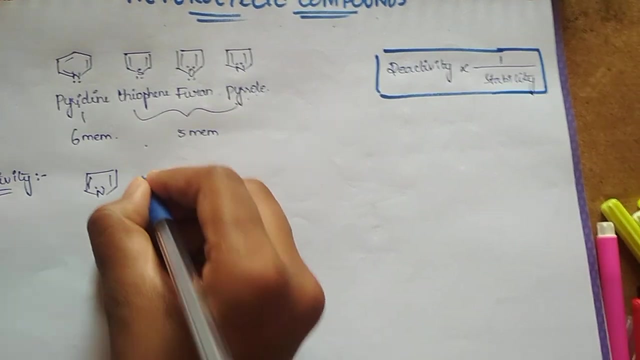 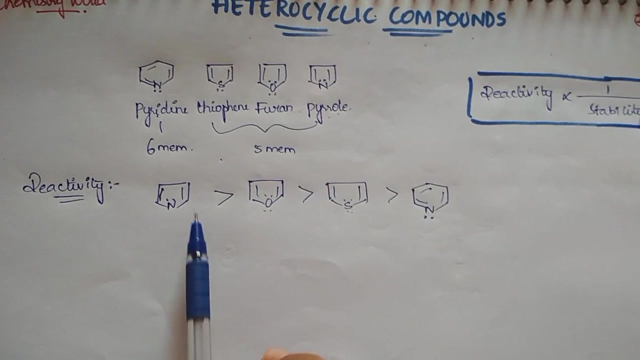 Reactivity is always inversely proportional to the stability. Okay, students, Okay. So, therefore, which is more reactive in this Pyrrole? More reactive? Okay, this is the order. First is pyrrole, Next furon, Next thiophene And next pyridine. 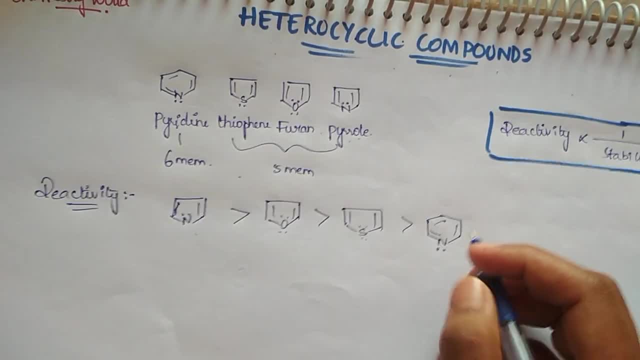 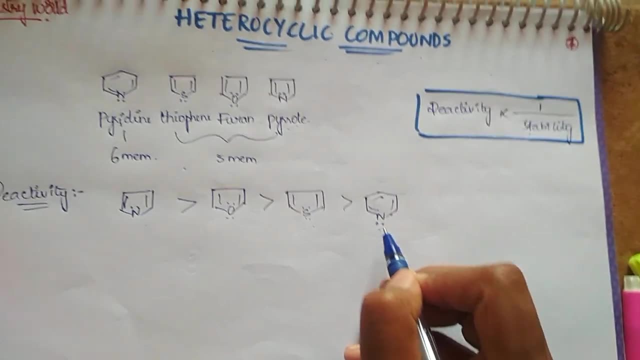 So pyridine is a six membered ring Right, So it is more So it is more So. pyrrole is more stable than these five membered. So more stable means what Less reactive. So we consider this as last So least reactive. 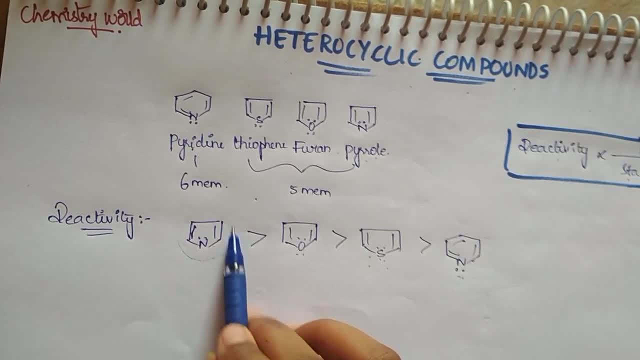 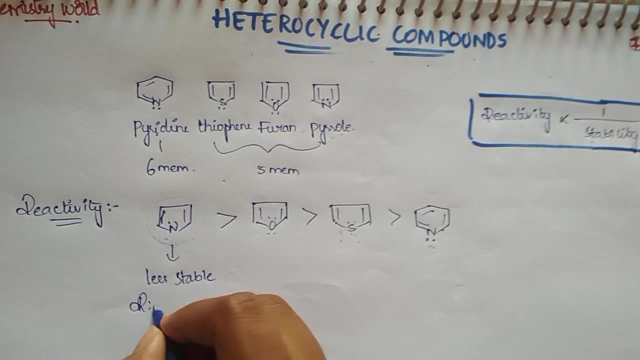 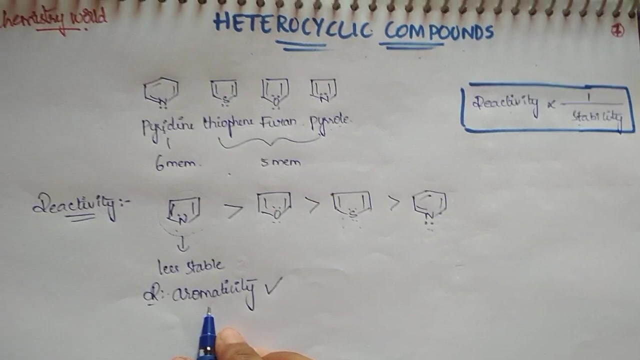 Based on the three, five membered rings we have, pyrrole is the most reactive due to the less stable. Why it is less stable Reason? it exhibits aromaticity perfectly. Most Okay, students, It is a major. So we have the trick here. 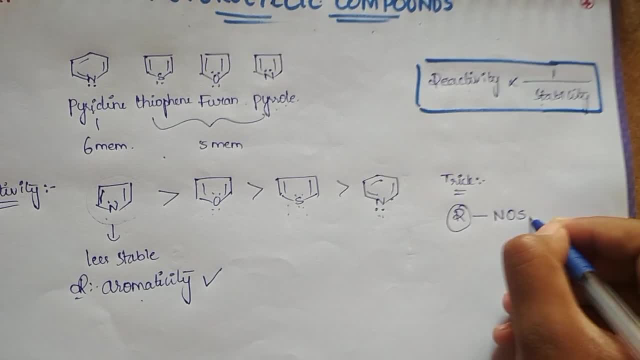 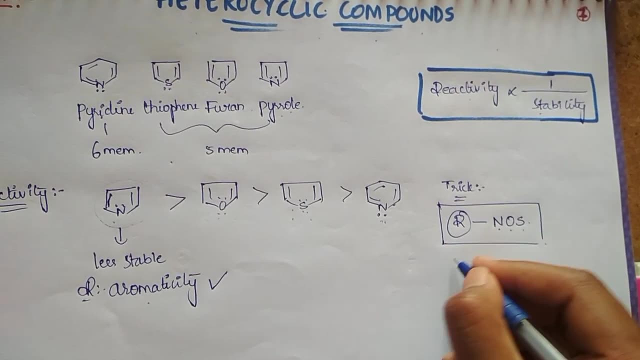 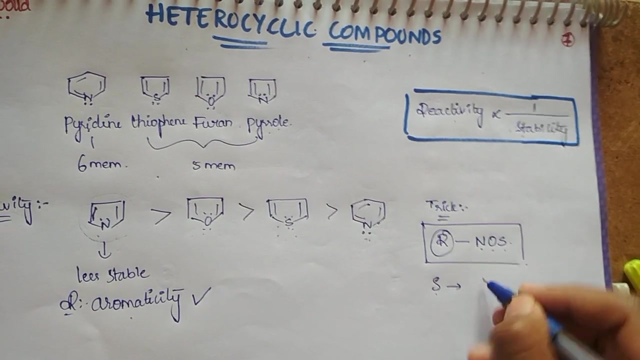 For reactivity order nos pyrrole, furon, thiophene. Okay, students, So the stability, what will become the reverse of the reactivity, is called stability right. So the stability order is S O N. 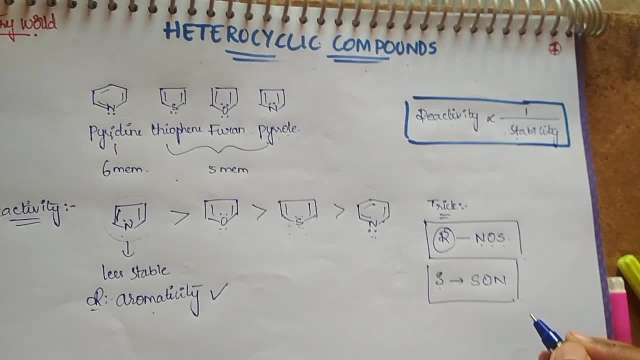 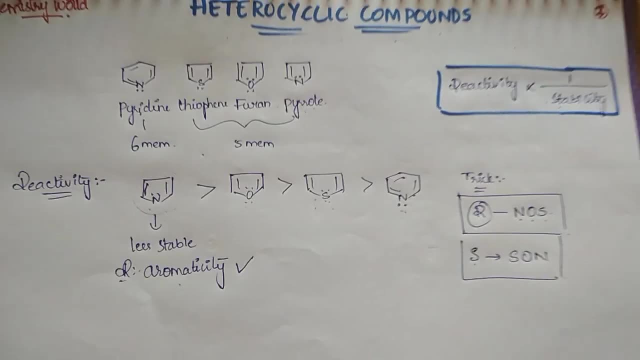 Sun. Okay, students, And this is the trick for you. Okay, students, And the time. Thanks for watching. Keep watching and if you have any queries, ask me in the comment section. Thanks for watching.